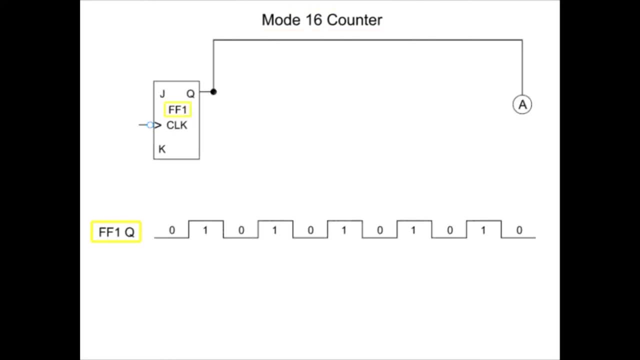 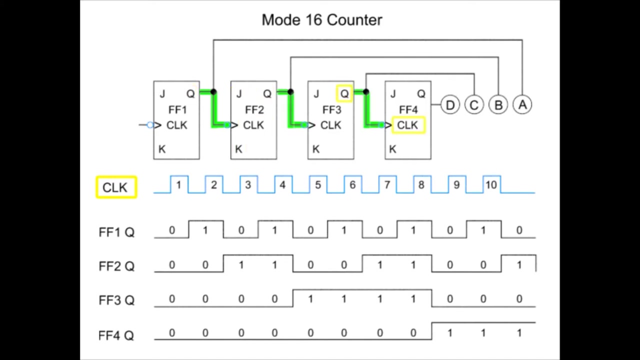 A Mode 16 counter uses four JK flip-flops as diagrammed here. In this circuit, the output at Q becomes the clock input for the next JK flip-flop. Each JK flip-flop is open. thus they are set automatically to high or 1,, which keeps them in their toggle position. 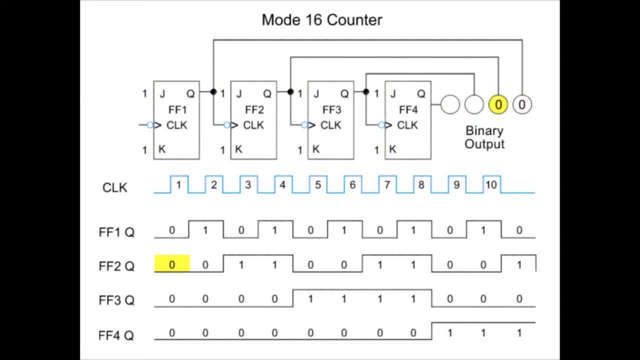 The counter starts at 0, 0, 0, 0.. As pulse 1 arrives at the clock input at flip-flop 1,, it toggles on the negative edge. The output at Q1 will go from low to high or 1, thus the counter will be at 0, 0, 0, 1.. 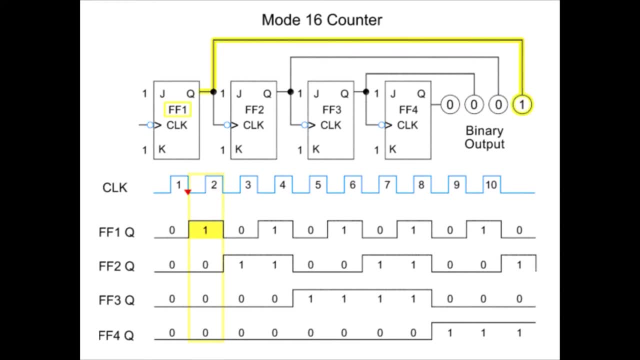 When clock pulse 2 arrives at flip-flop 1,, it returns output Q1 back to 0, which causes flip-flop 2 to toggle to 1.. The output at Q2 is 1, and the count on the display now reads 0, 0, 1, 0.. 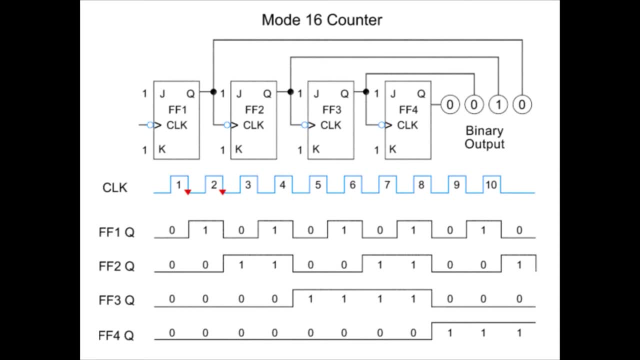 The counting continues with each flip-flop output, triggering the next flip-flop. on its negative going pulse, The 1's position, or A, must change its state on every count. Thus flip-flop 1 must toggle for each clock pulse. 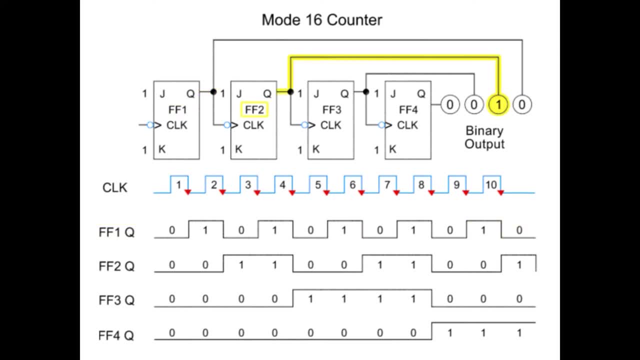 The 2's position will change its state half as often as the 1's position. Thus, flip-flop 2 will only toggle half as much as flip-flop 1.. The 4's position will change its state on every count. 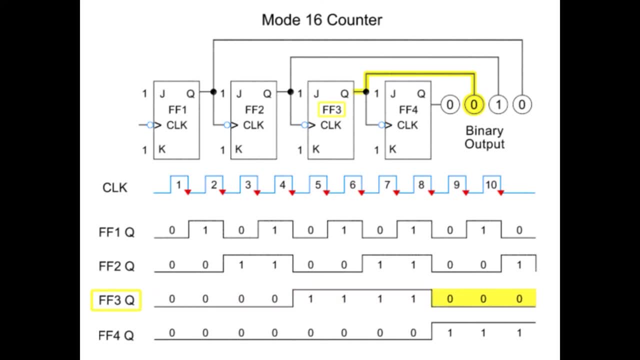 Thus, flip-flop 2 will change less often than the 2's position and the 8's position less often than the 4's. Thus, each more significant bit will toggle fewer times. Let's observe how a sequence of 10 clock pulses will ripple through a series of 4 flip-flops in this 4-bit counter. 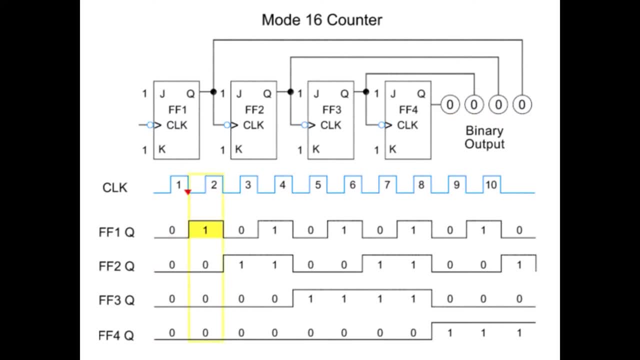 As we have shown, the first clock pulse generates a binary output of 0, 0, 0, 1, and the second an output of 0, 0, 1, 0.. As the remaining pulses arrive at the input, 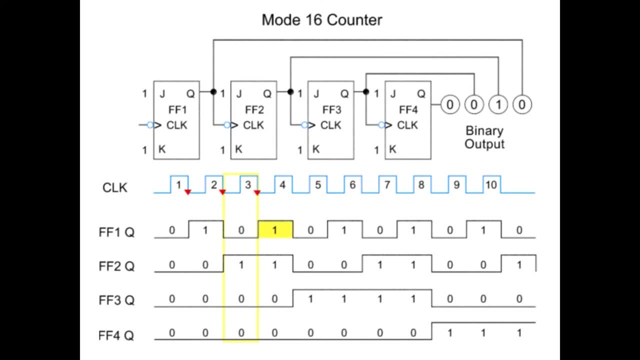 the third pulse toggles Q1 back to 1,, with Q2,, Q3, and Q4 remaining unchanged, and the output is 0,, 0, 1, 1.. Pulse 4 again toggles Q1 back to 0,. 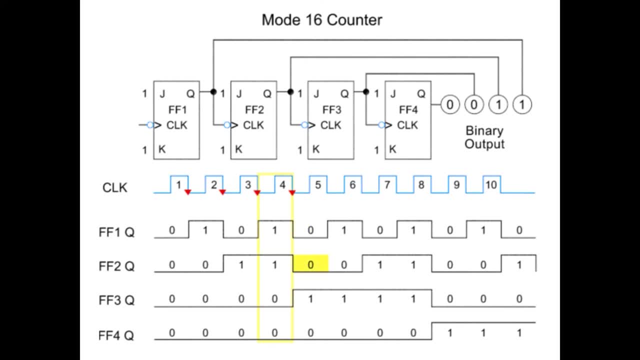 with Q2 toggling to 0, and Q3 to 1, with Q4 unchanged, and the output is 0, 1, 0, 0.. These toggling patterns triggered on the negative edge of the clock pulse. 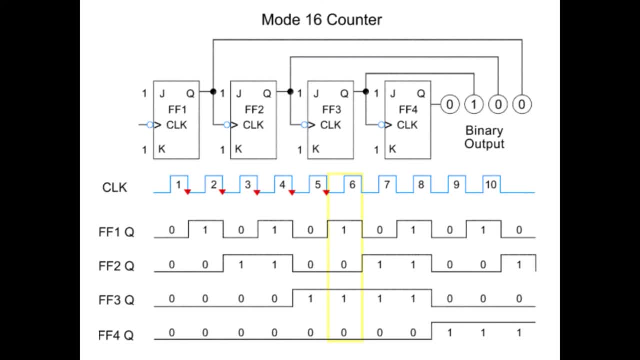 continue with pulse 5, giving an output of 0, 1, 0, 1.. Pulse 6: outputs 0, 1, 1, 0.. Pulse 7: outputs: 0, 1, 1, 1.. 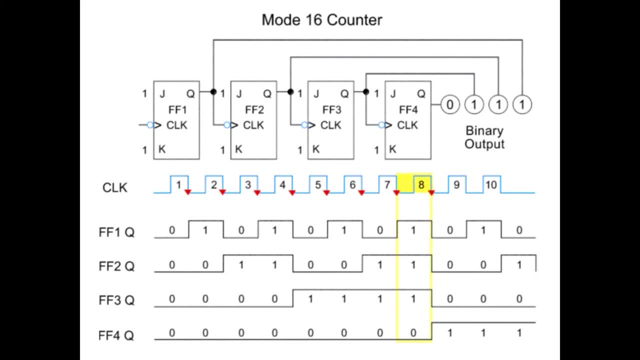 The 8th pulse results in an output of 1, 0, 0, 0.. Pulse 9, a 1, 0, 0, 1.. And finally, as expected, the 10th pulse. 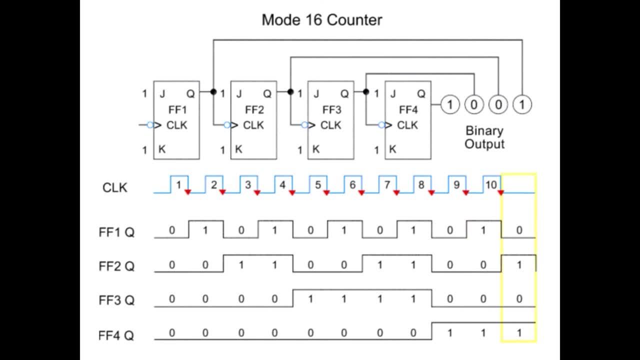 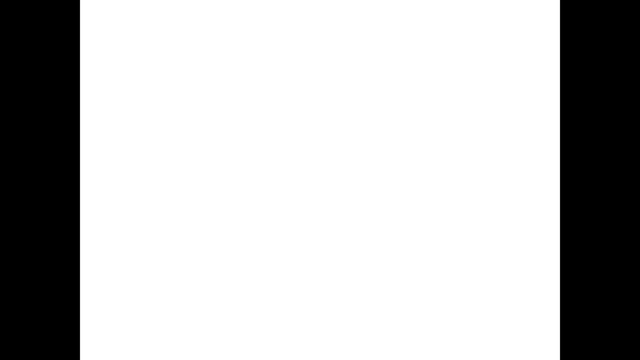 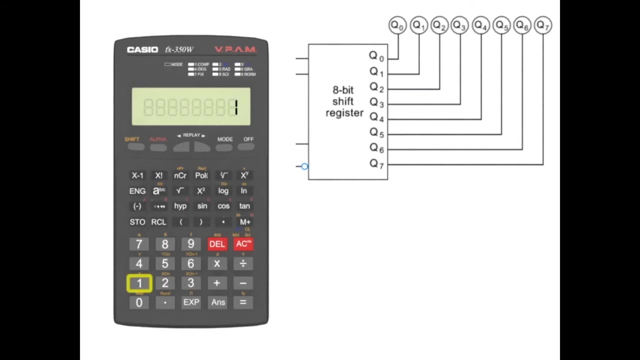 toggles the appropriate flip-flops to give 1, 0,, 1, 0.. The digital memory, storage and bit-shifting characteristics of the shift register is essential in many digital electronic systems. The keying of numbers into a calculator demonstrates the practical application of a shift register. 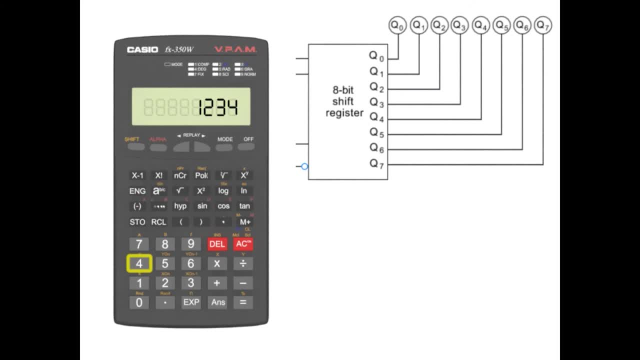 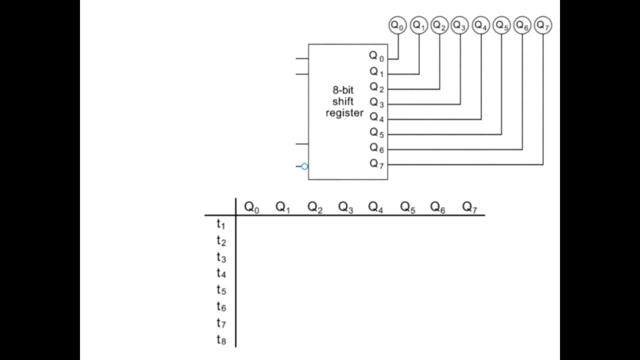 As numbers are entered, they are stored and displayed. Each subsequent number that is entered shifts the previously entered number to the left. Let's look at how a shift register operates by observing the shifting of an 8-bit register based on a series of binary data inputs. 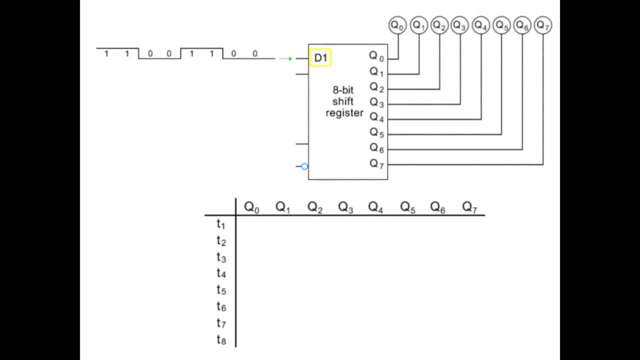 We have two serial inputs, D1 and D2, arriving at an AND logic gate, A master reset input at MR which, when activated by a low or zero input, will override all other inputs and reset the Q1 through Q7 outputs to zero. 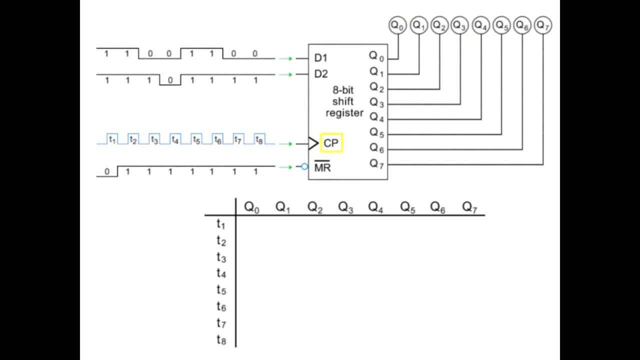 A clock pulse input, CP, which will be enabled when transitioning from low to high. The right-pointing triangle symbol without the bubble signifies this clocking functionality. Let's input the binary data at D1 and D2.. With an AND gate when both inputs are high. 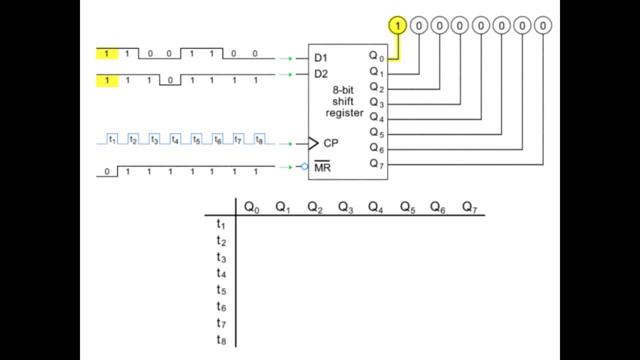 the output is high and, conversely, when either inputs are low, the output will be low At T1, the zero or low at MR overrides the D1 and D2 inputs and sets all outputs to zero At time T2, D1 and D2 are high or 1.. 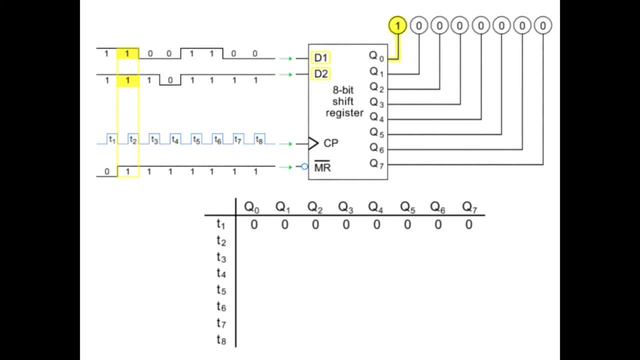 Thus the output at Q0 is 1.. This information bit is placed in the Q0 position in the register. This shifts the other bits one place to the right At T3, the input of zero at D1 and 1 is high. 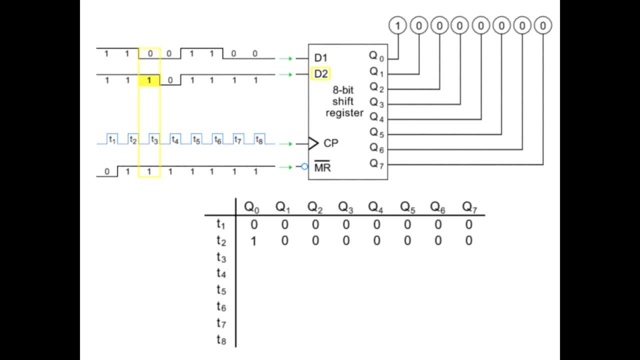 and conversely, when both inputs are low, the output is low and conversely, when both inputs are low, results in an output at Q0 of zero. The zero at Q0 replaces the one again, shifting all the bits one position to the right. 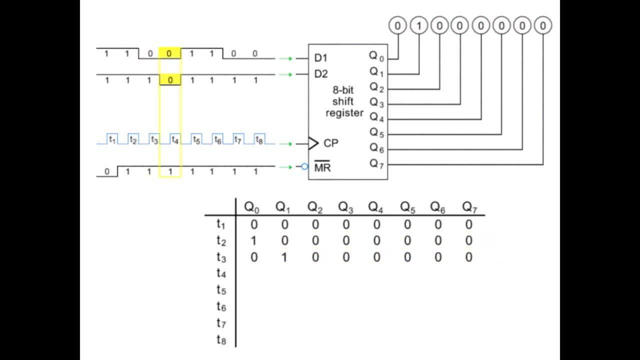 The zero and zero input at T4 again outputs a zero, which drops in to the Q0 position. shifting the bits again to the right to the right At T5, the input of 1 outputs a 1 that drops into the Q0 position.